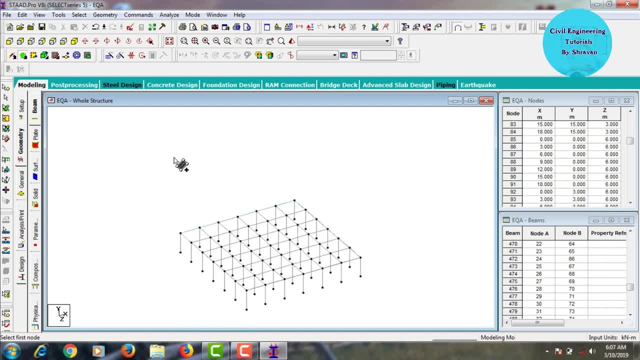 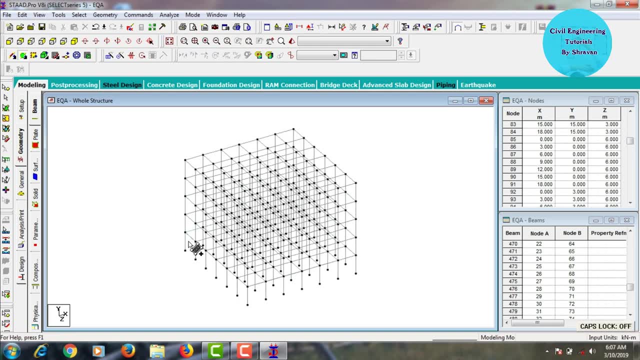 Ok, So it was assigned with node plate. So now go to close structure command. Now we need to copy the whatever the slab section is there in our first story we need to copy to the remaining見 stories. for that: go to select your plate. cursor. select your plate. go to transitional. repeat in. 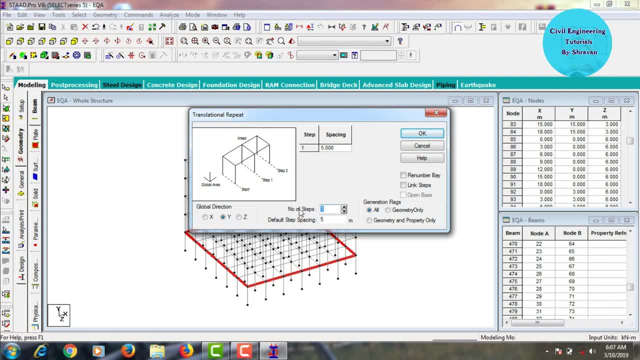 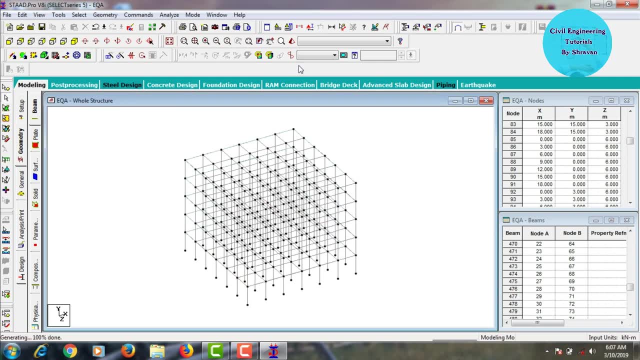 y direction. so number of steps- just we need to assume number of steps are 4- each step will be consisting of 3 meter height. click on ok button. now i will show you this model in 3d view. this is my 3d view of the respective building. so now we need to apply the member properties, nothing but. 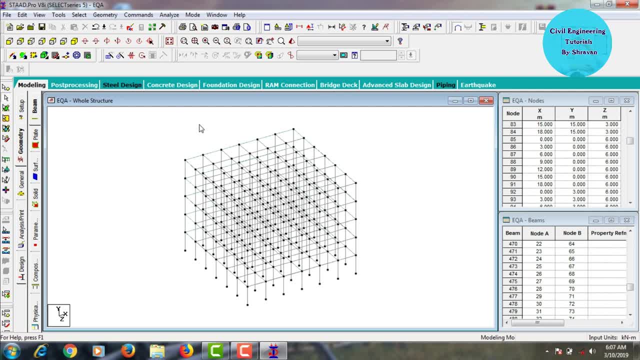 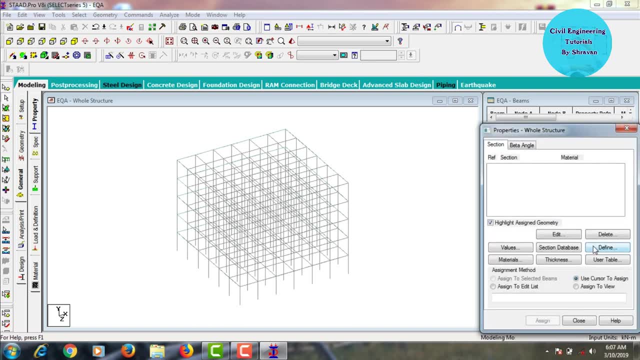 beam sizes, column sizes, as well as slab thickness for the respective building. for that go to general. so go to click on property. here we need to define the beam size, column size for the respective building. click on define button. go to select your rectangular. so just, i am assuming the beam size of 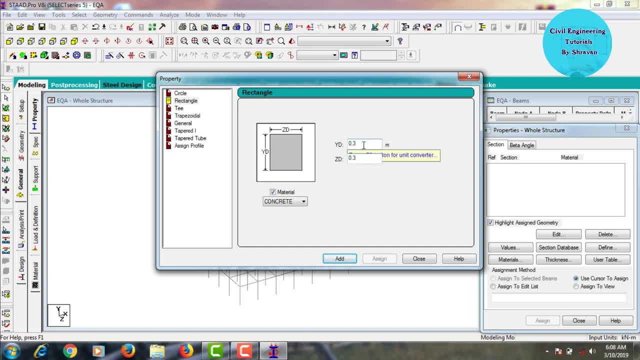 0.3 meter by 0.3 meter for the respective d plus 4 building. just add it after that. just i am assuming 0.45 and 0.45 is my column size. so after that i will show you the 3d view of the respective building. 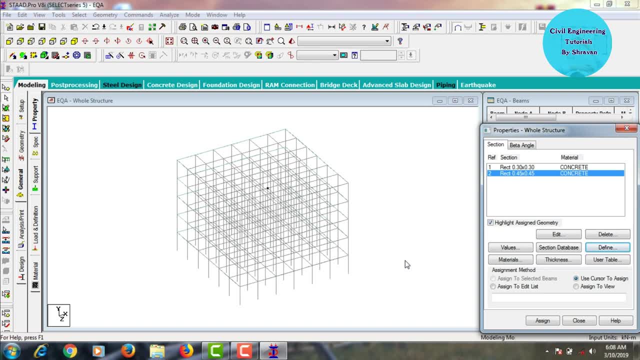 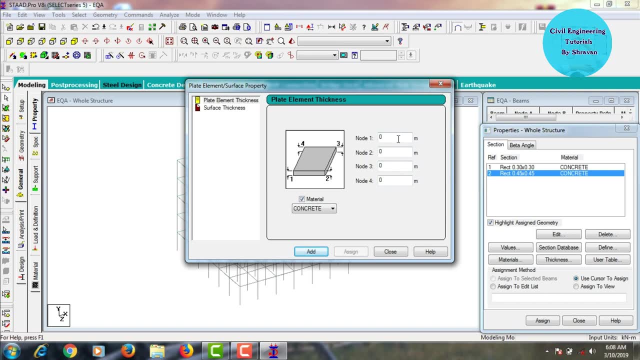 just close it. now we need to define the slab thickness for the respective building, so for that you need to click on the thickness here. so here, node 1, node 2, node 3, node 4 is there. so just, i am assuming the node value value of thickness is 0.125, nothing but 125 mm. just add it, just close. 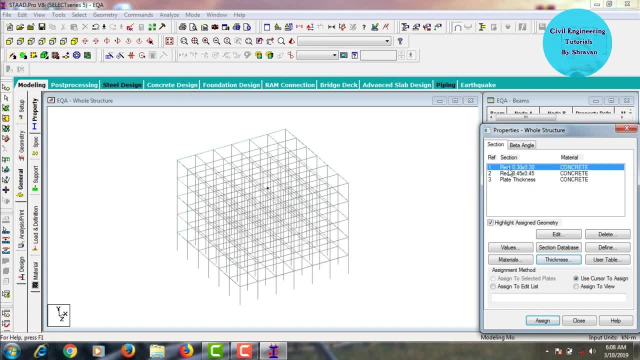 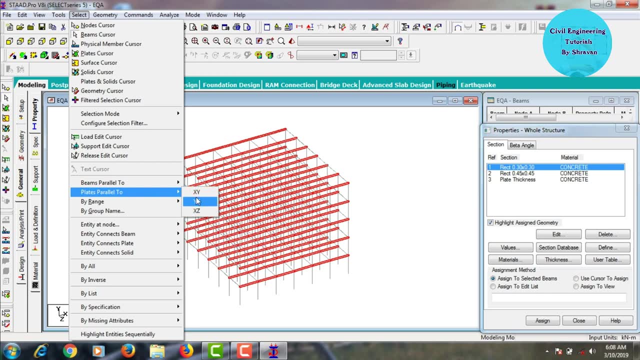 it now. select your rectangular: 0.3 by 0.3. this is nothing but your beam. go to select option: beams parallel to x direction. again go to select option. beams parallel to x direction. again go to select option: beams parallel to z direction. click on. assign to selected beams here. click on. 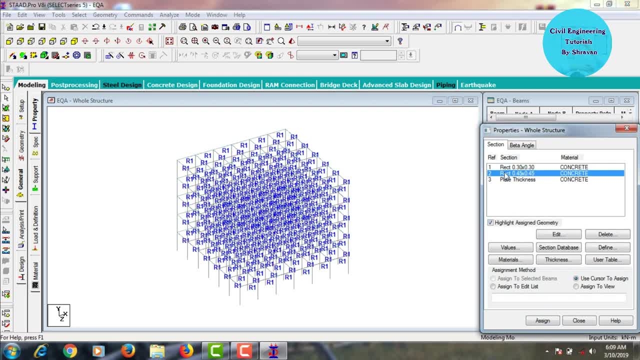 assign button. click on s button. so after that select your 0.45 by 0.45. so this is nothing but your column. go to select beams parallel to y direction. okay, click on assign to selected beams. assign yes. now go to select your plate thickness. click on assign to view. assign- yes. now go to 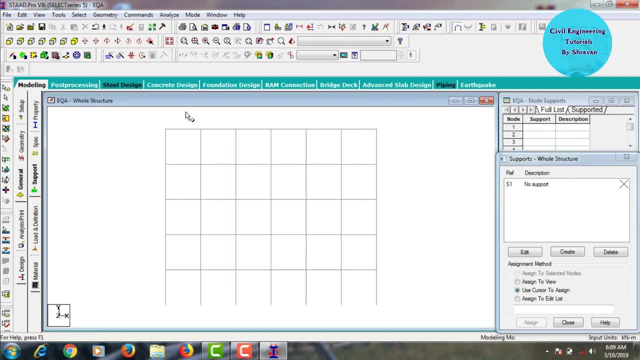 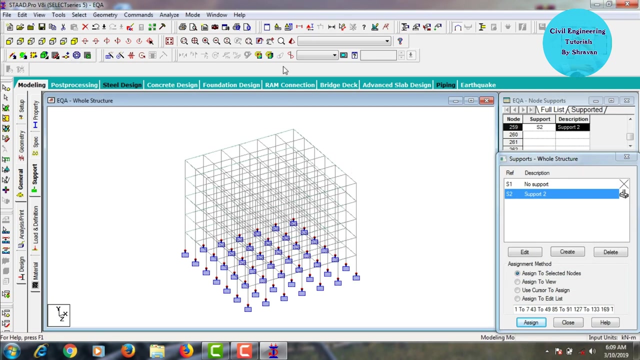 supports. keep your structure in front view. click on create button for creating fixed support. just add your fixed support. select your support to nothing but fixed support. now select your node point at the bottom section. now click on assign to selected nodes: assign. yes, now i will show you this model again in 3d rendering view. this is my 3d. 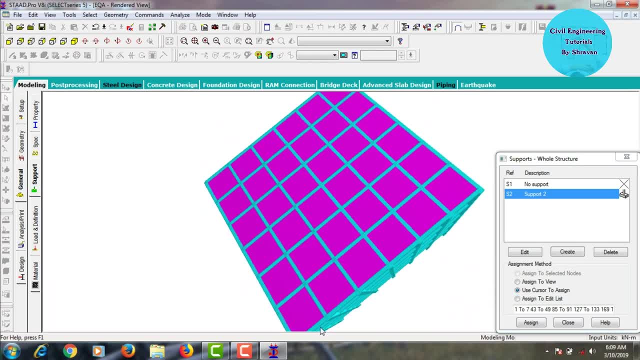 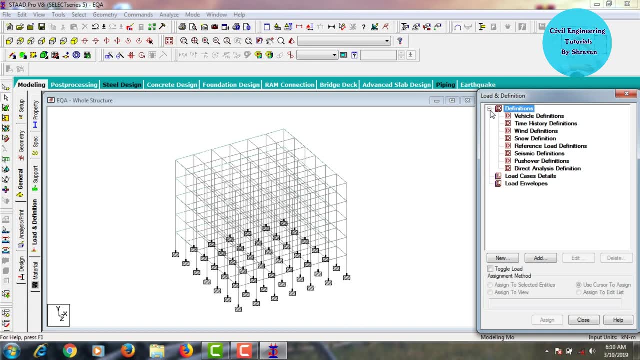 rendering view for the respective g plus 4 building. now, after that, go to loads and definitions. in order to add your seismic load in load case details, initially we need to define the seismic loads, so for that click on loads, definitions, values plus 1, so in this we need to select seismic. 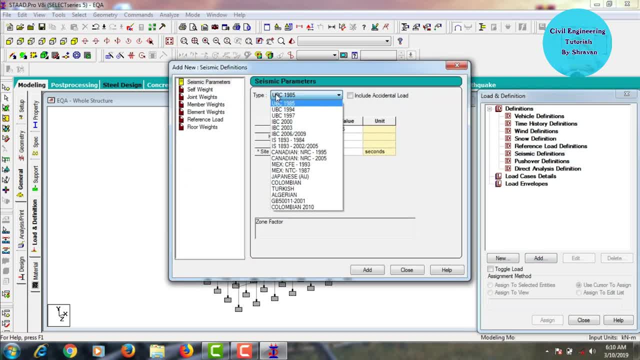 definitions: click on add button. so here here we have type. type is nothing but code name. so here we have number of codes. so in this code just time i am considering is 1893, 2002 by 2005. just click on that. okay, here we have one, two more, uh. 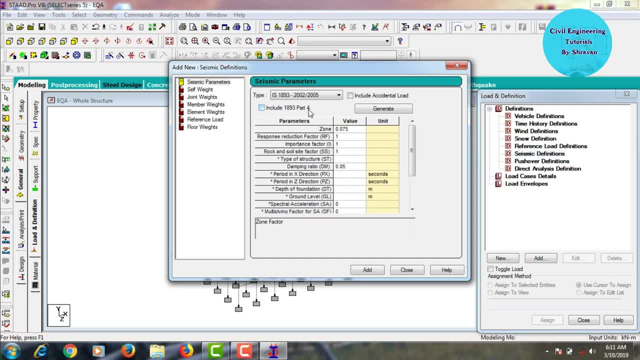 include 1893 part 4. so this 1893 part 4 code will be helpful for designing of industrial structure or steel building. if you are designing industrial structure or steel building, just you need to select this tick mark, otherwise please ignore this code. so include accidental loads. 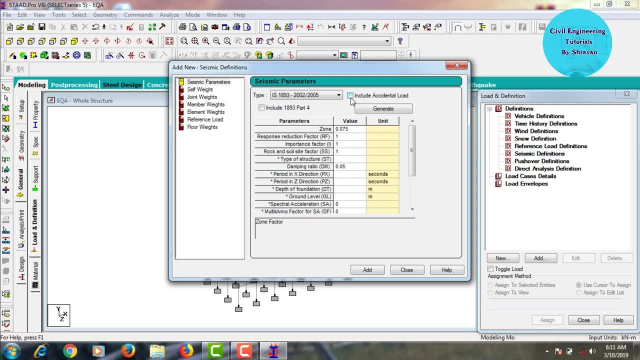 so accidental loads: if you have any accidental loads in your building, just select this option, otherwise leave it. so go to click on generate button. so here we have already defined some values. so, but as per our assumption, we need to define the seismic load values. so for that, click on generate button. 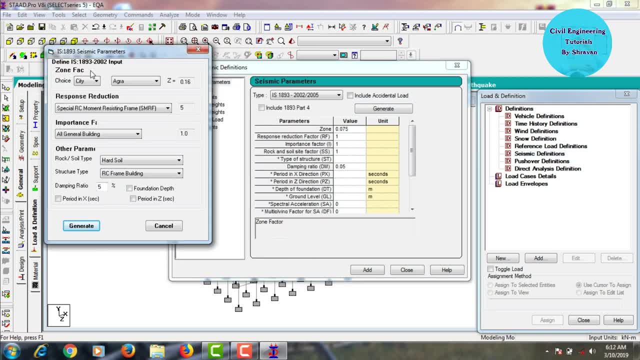 as per IS18 entry 2002 code was divided seismic zones into 4 categories: zone 2,, zone 3, zone 4, zone 5. so zone 2 will have value of Z value as 0.10. zone 3 will have is a value of 0.16. zone 5 is having 0.24 and zone 5 is having 0.36, so zone 2 comes under low seismic zone, zone 3 comes under medium seismic zone and zone 4 comes under high seismic zone. so zone 5 is severe case. 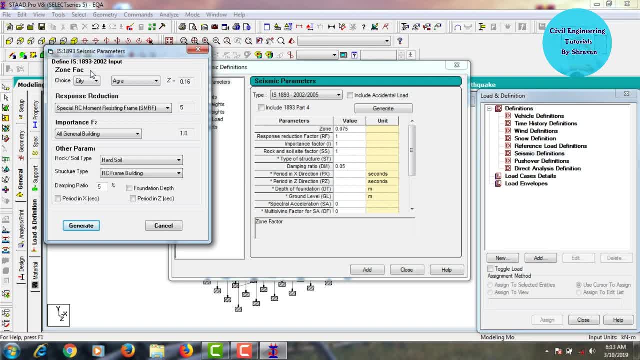 so for this building, just I am considering the severe case. so here, choice type. so we have two types of options here: city or zone. if you know the city name, just select your city or else go with zone. so just I am going with the zone, select your zone. 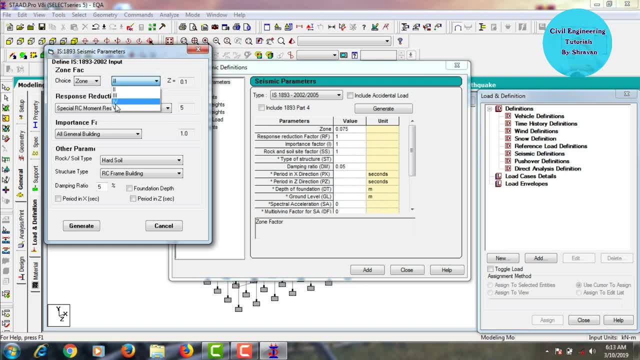 so here, just I am selecting the zone 5. zone 5, so it is having factor of 0.36. so here, response reduction factor. these are the different types of building. so here for the respective G plus 4 storey building, just I am considering. 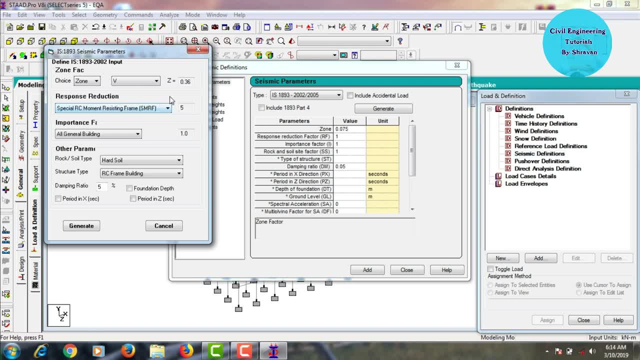 special RC movement resisting frame building. so width 5 is the response reduction factor. so after that we need to enter the importance factor. so for the respective importance factor, we have important building as well as all general building. ok, so I am selecting here as all general building. 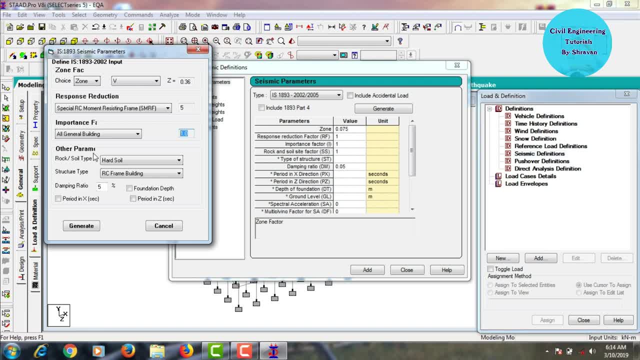 with importance factor as 1. so here other parameters, nothing more. rock or soil type, so here I am assuming the medium soil. so medium soil, select your medium soil. so structure type: RC building, steel building, frame building, other building. so here it is: RC building, select your RC building. 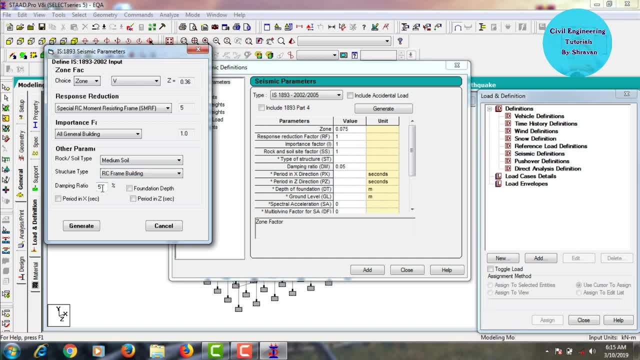 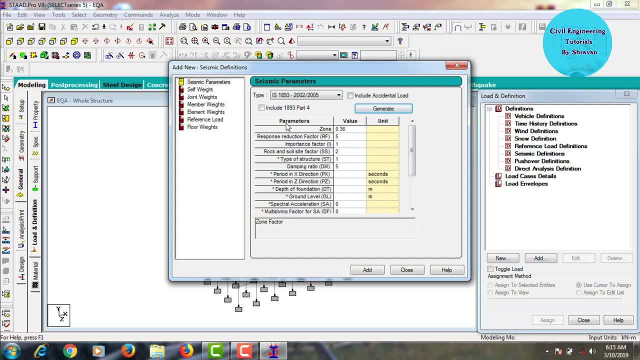 ok, so here damping ratio: for any building we need to consider 5 percentage of the damping ratio. so click on generate button. so here it was generated. the values, parameters, values, units. so zone value: 0.36. response reduction factor is 5. importance factor is 1. 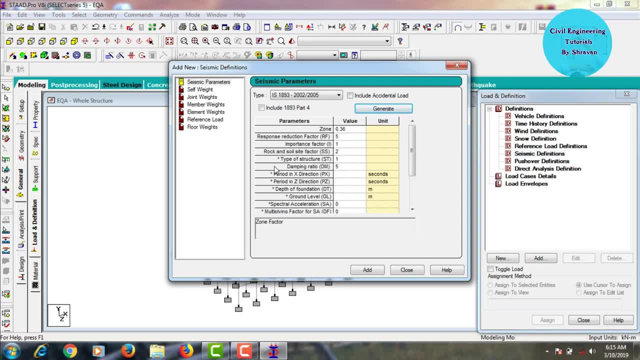 soil type is 2. nothing but medium soil. type of structure is 1. damping ratio is 5. so here we need to change this 5 from 5 to 0.05. now click on add button, so here we need to add the self weight of the building. 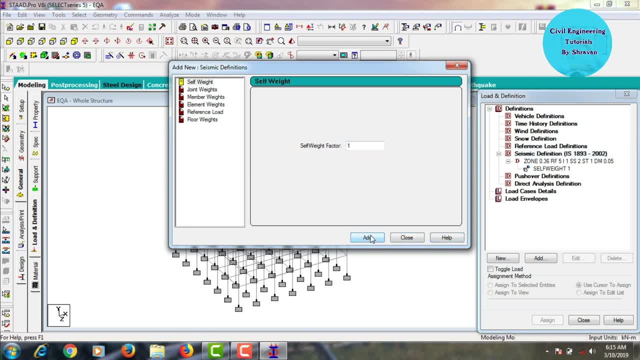 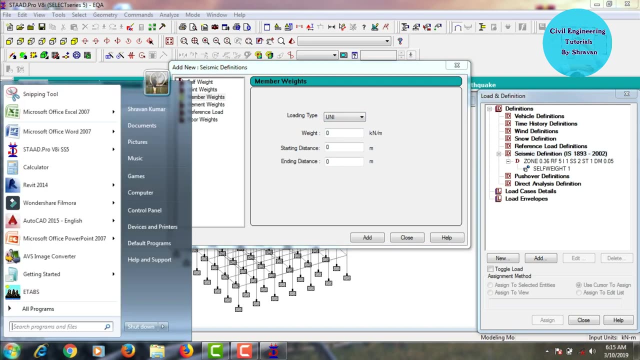 initially we need to add the self weight of the building, so after that we need to add the member weight. member weight. so in this load type we need to select the concentrated load to uniform load, so U and I. so here we need to enter the values. this value can be calculated by using the dead load of the beam. 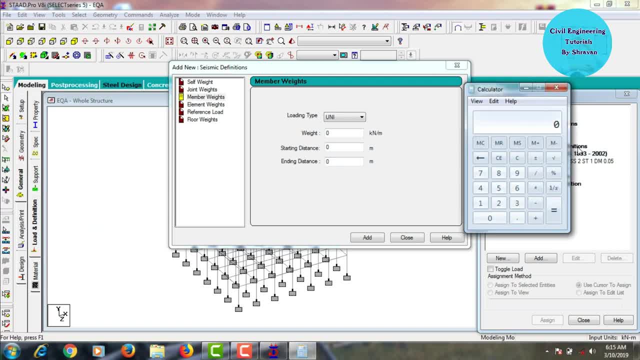 so I am calculating now. I am calculating the dead load of the beam. my beam size is 0.3, cross 0.3. we need to multiply this by unit weight of the concrete. 25 will give you 2.25. so minus is the downward direction. 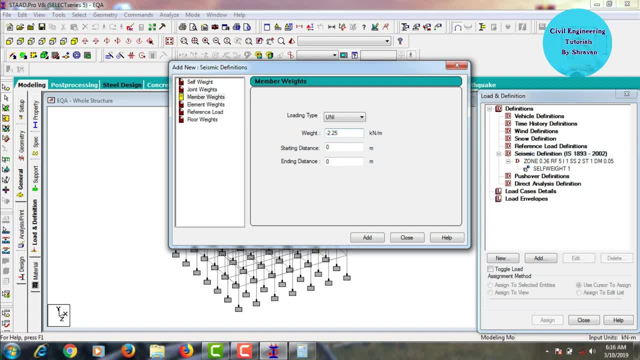 so minus 2.25 is the value of uniform load. just add it. so after that we need to add the floor load for the respective building. so floor weights: click on floor weights. so we need to calculate the floor weights also for the respective building by using the thickness of the slab. 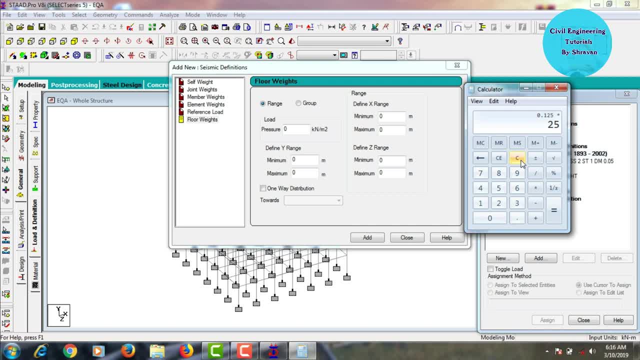 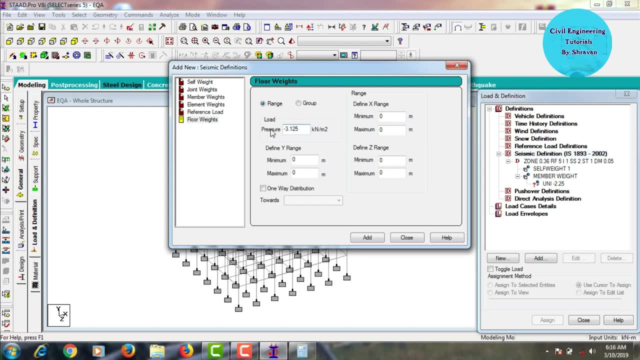 and multiplied by 25 unit weight of the concrete will give you 3.125, is the floor weight minus 3.125. so my first slab is at 3 meter as well as my last slab is at 15 meter. so y range is 3.25. 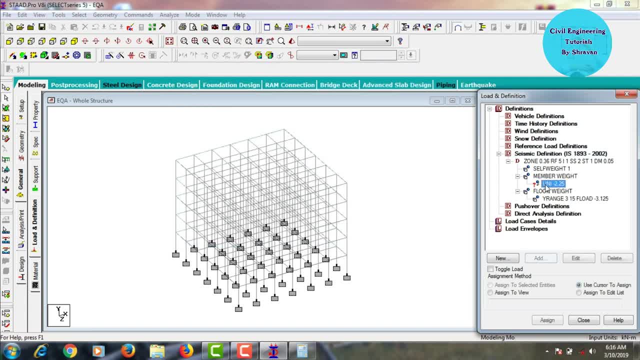 that means I have added 25 to 15, just added this floor weight. now select your uniform load of minus 2.25. so we need to apply the uniform load of 2.25 for the beams. so for that case we need to select the beams. 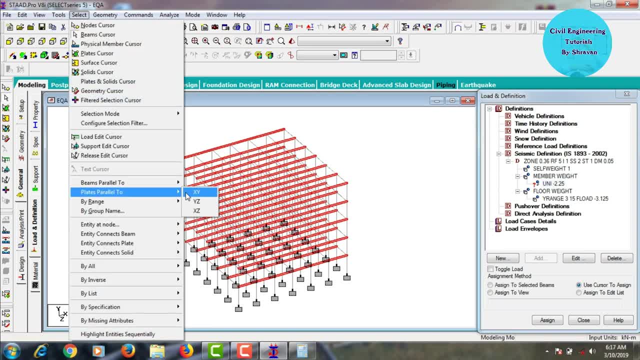 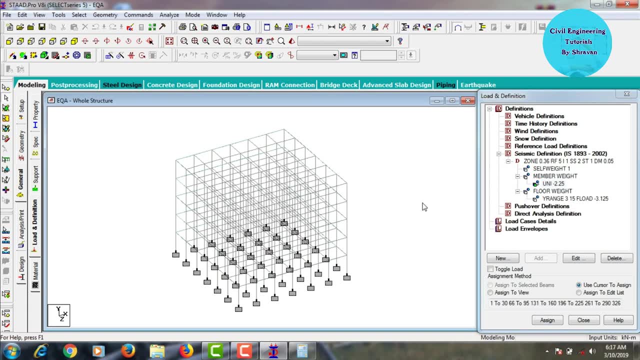 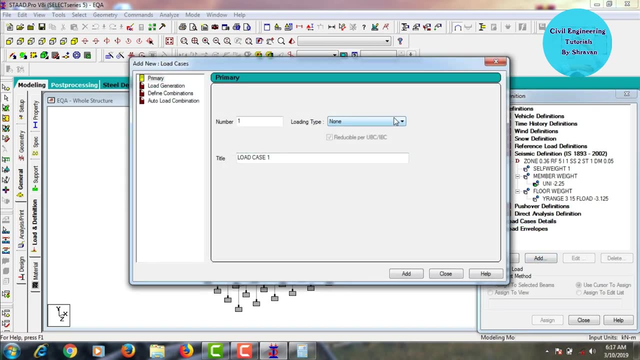 parallel to x direction. go to select and select beam. parallel to z direction. now click on assign to selected beams and assign yes. so after this, go to load case details. click on load case details. click on add button. need to select the load type. so just, i'm selecting here a load type as seismic, so here we need to. 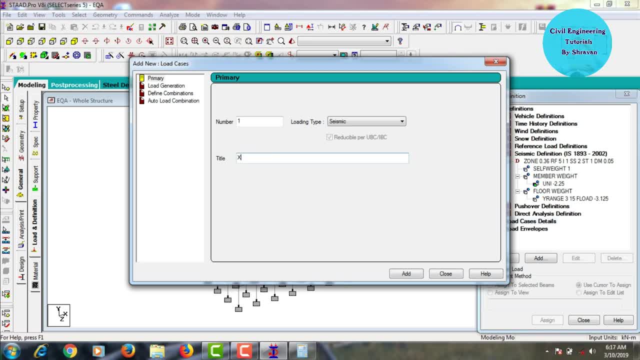 enter the load title is: earthquake load in x direction- just add it. after that: earthquake load in z direction- just add it. earthquake load in minus x direction: add it here also. we need to add earthquake load in minus z direction. add it now. just cancel this. go to x. just click on add. 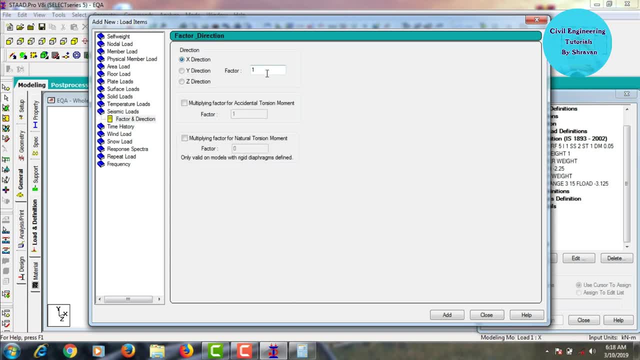 button. here we need to select the seismic load. so x direction with factor of 1: just add it. close it now. go to select your z: just add it now. go to select your seismic loads in z direction with the factor of 1: just add it. close it. now select your minus x: click on add button now select your. 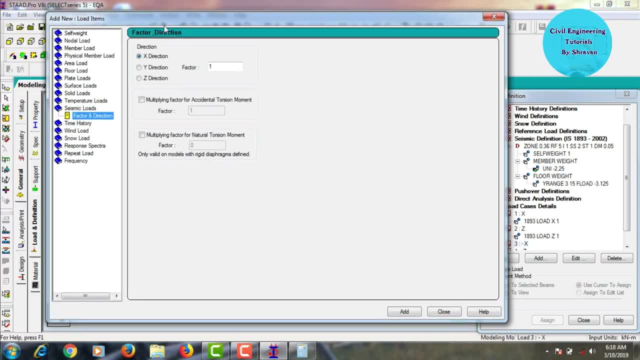 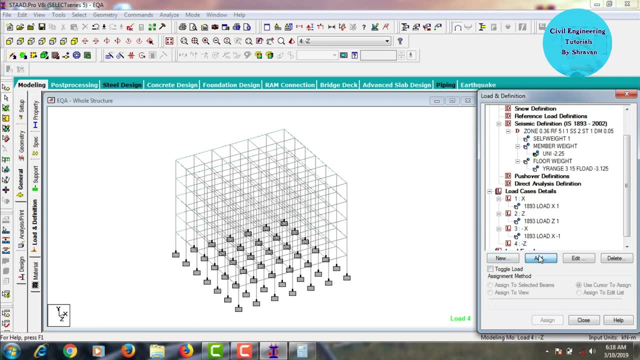 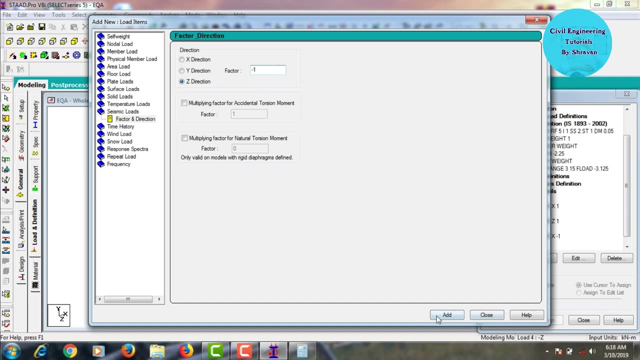 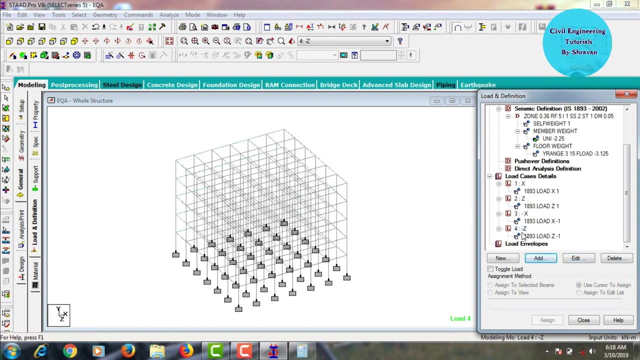 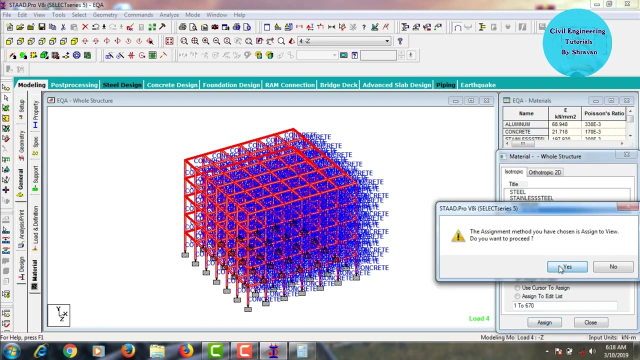 seismic load here, so in x direction. so with factor of minus 1, add it. after that, go to select your minus z. just click on add button. Now select your seismic load in Z direction. minus 1 is the factor. So 1 is from left to right side, minus 1 is from right to left side, in the same way for the respective Z direction. Now go to materials. select your concrete. click on assign to view. assign. yes.